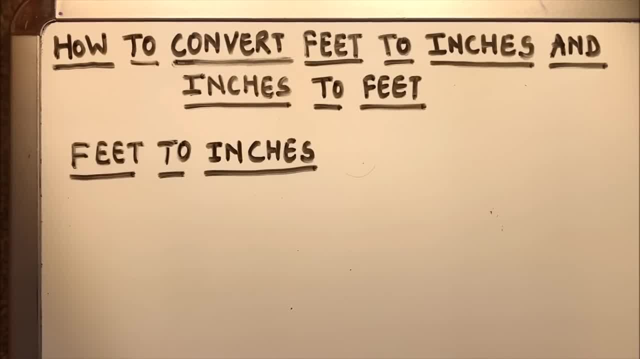 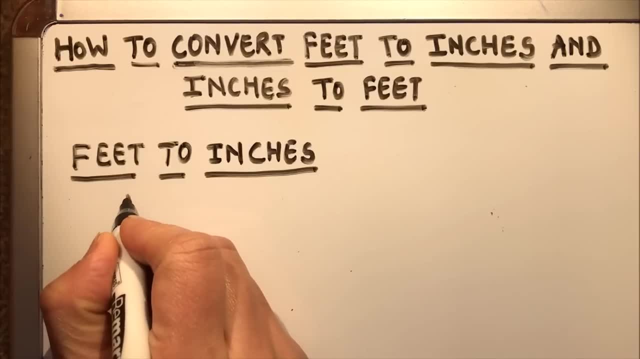 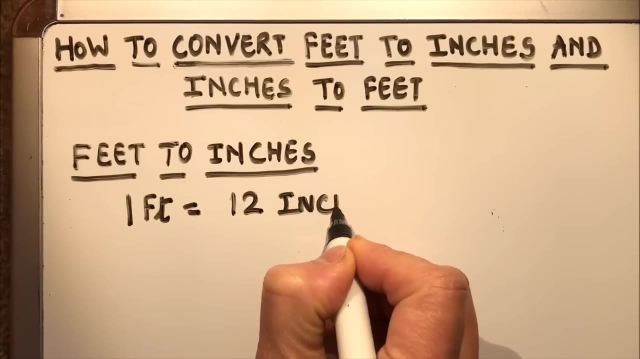 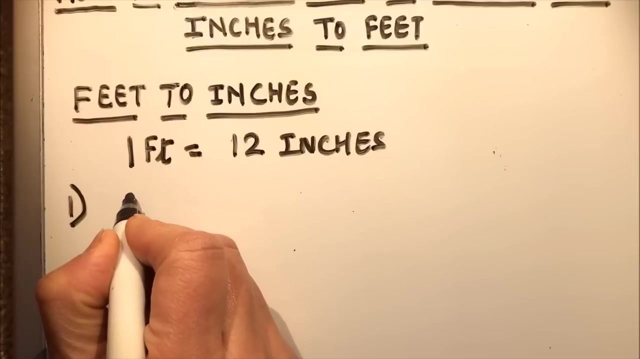 Hello viewers, today we are going to learn how to convert feet to inches and inches to feet. So first of all we will do feet to inches. So, as we all know, that 1 feet is equal to 12 inches. So if we need to find out how many inches are there in 7 feet, 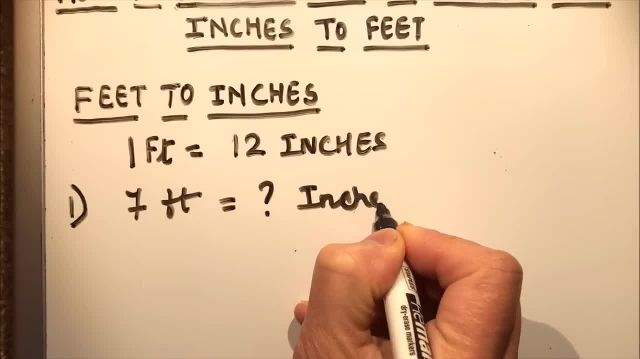 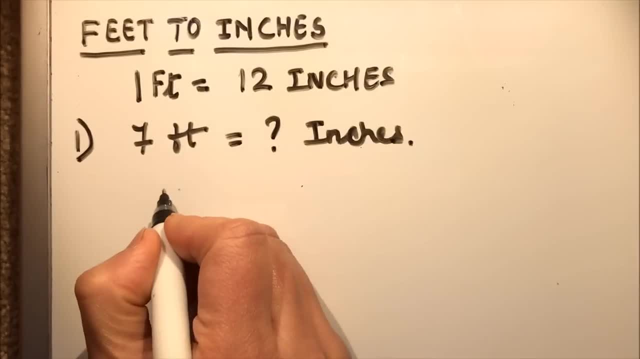 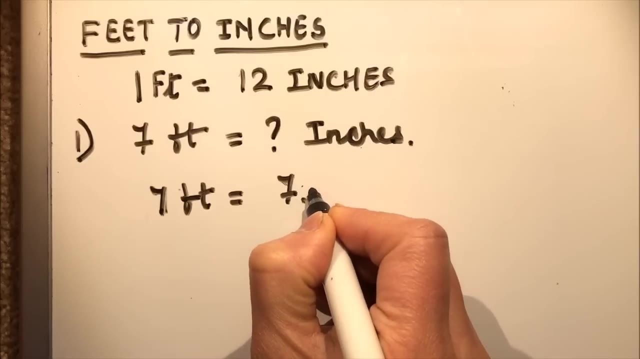 So from the above relation we know that 1 feet is 12 inches, So 7 feet is. we can write 7 feet as 7 multiplied by 1 feet. So what we will do now that we will put the value of 1 feet in terms of inches here. 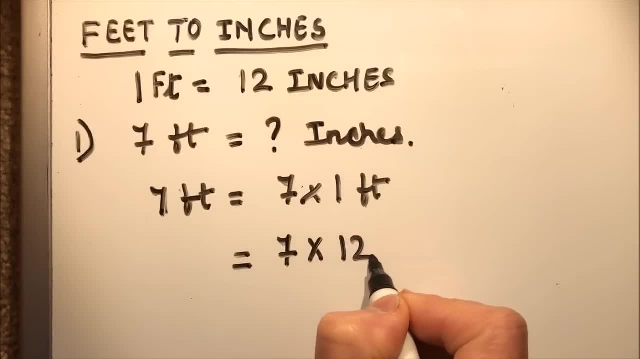 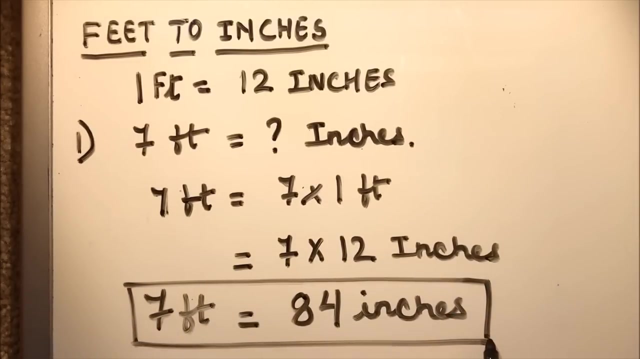 So 7 feet is 7 times 12.. So this is going to be: 7 times 12 is 84 inches. So this is how we can convert feet to inches. So now we will move to the next thing, which is to convert inches to feet. 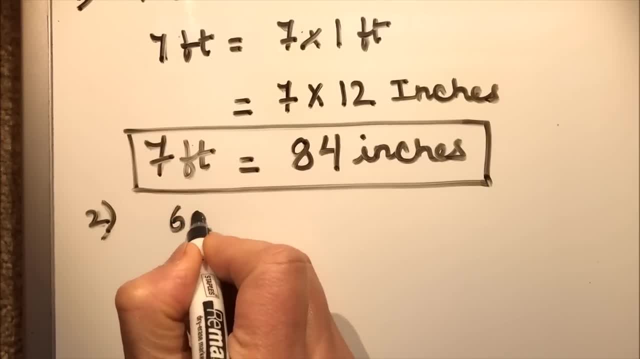 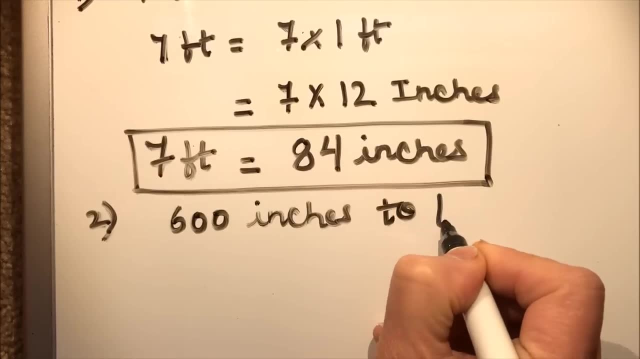 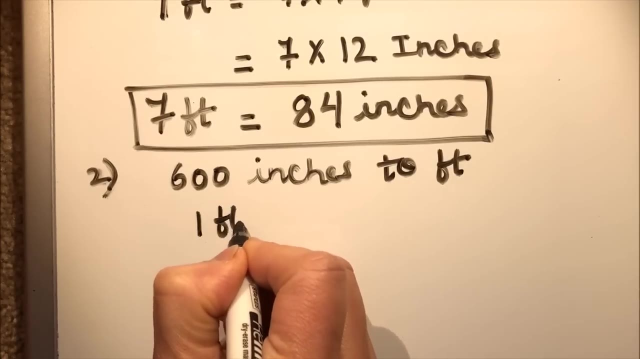 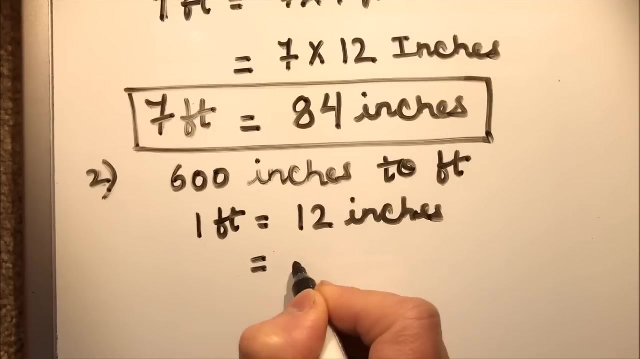 So I have a question To convert. To convert 600 inches to feet. So what we will do. we all know that 1 feet is 12 inches, Or we can write it as 12 times 1 inch. 1 feet is 12 times 1 inch. 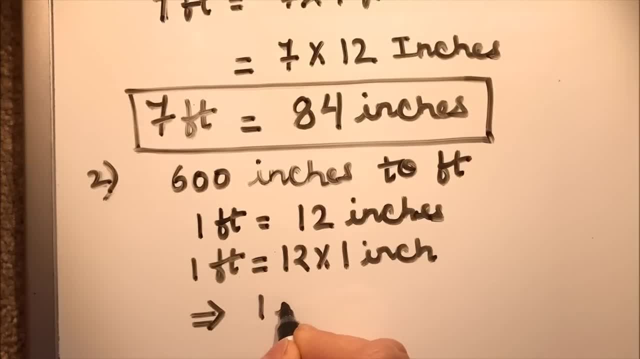 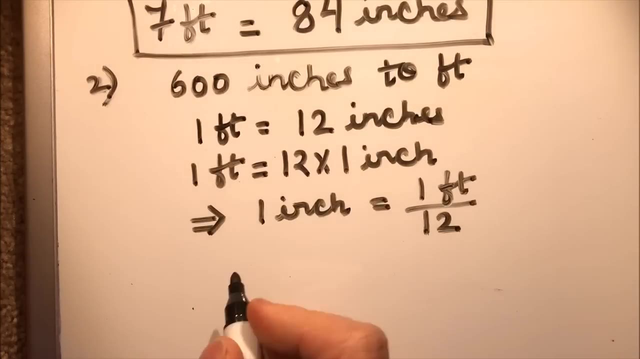 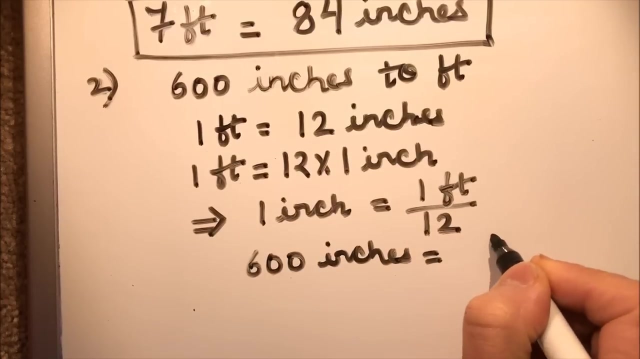 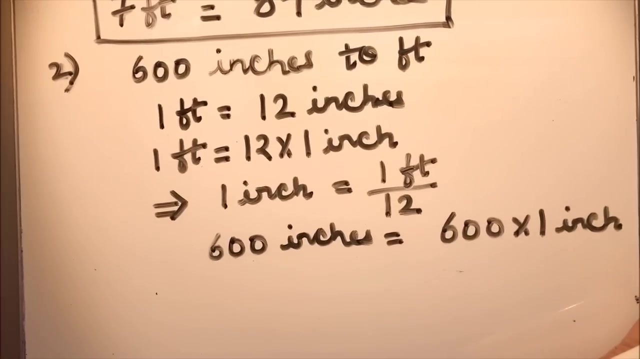 1 inch, which gives us that 1 inch is equal to 1 feet over 12.. So we all know that 1 inch is 1 feet over 12.. So 600 inches, we can write 600 times 1 inch. So now what we will do. we will put the value of 1 inch in terms of feet.